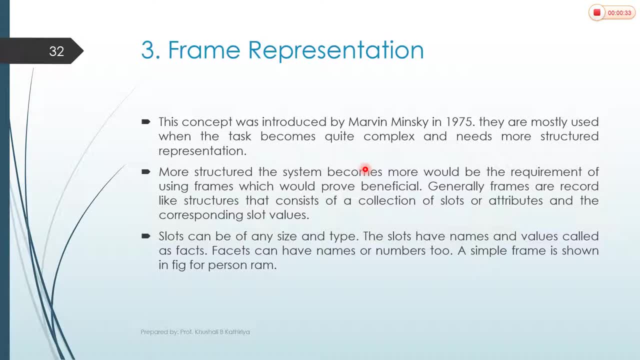 Or third approach is of knowledge representation. This is a frame representation. This concept is introduced by Marvin Mixie in a 94 or 1975. They are mostly used when the task become quite complex and needs more structure representation. Then they are used for frame representation. Then, when they have a quite complex problem, Okay, They want a more structure representation. 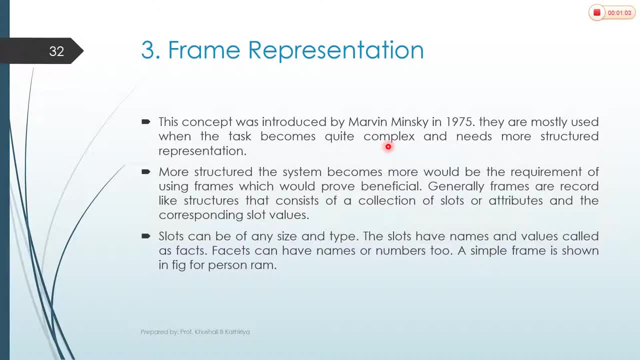 For the particular knowledge or particular data, then they use a frame representation. Okay, More structure the system. more structure system become more work be a requirement of using a frame with word proof beneficial. Generally, frame are recorded record like a structure that consists of the collection of slot or attribute and the corresponding slot value. Okay, So here our frames are. 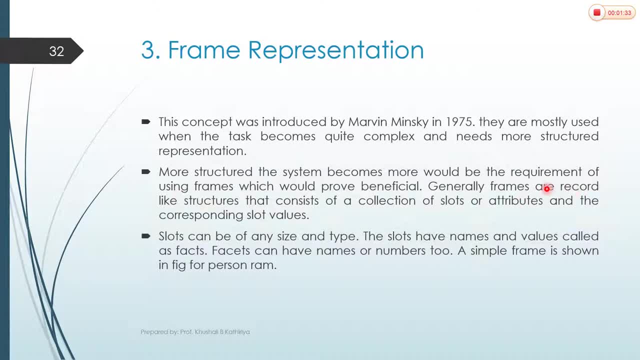 records like a structure. Okay, It is a use like a record. Okay, Frame is a use. Ah, Or frame are the records like a structure? Okay, Frame kya hai, Woh ek structure hai? And this is a collection of slot or attribute. Okay, Frame kya. 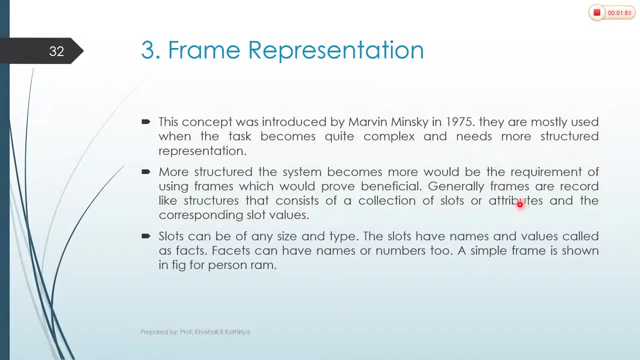 hoge Wo slot or attribute ka collection hoga Aur wo kya hai. Slot is a particular value bhi ho saktee. Okay, Slot can be any size or any type. Okay, The slot have a name and value called as fact. okay, here I have said frame are recorded like a structure. 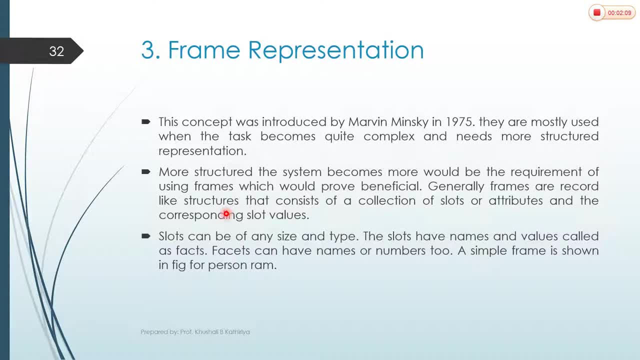 what we represent, frame in structure, we record it, we store it. that particular, whatever we store it, what we call it slot, we call it attribute and we call it value of its slot. and slot can be any size. okay, its value, its attribute, its name, its size can be anything. 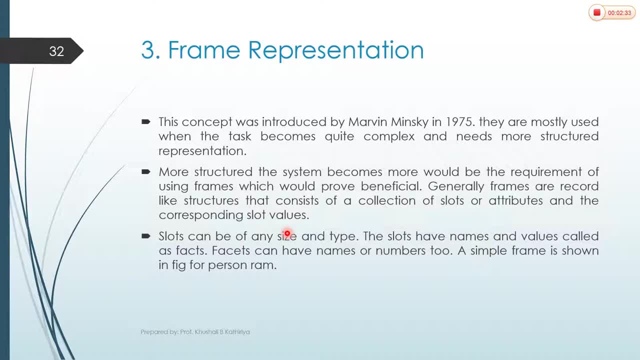 it can be any type, it can be any integer, it can be any number, it can be any digit. it means it is real number. it is real number, it is natural number, it is in alphabet. any integer character, any type can be this slot, have a name and. 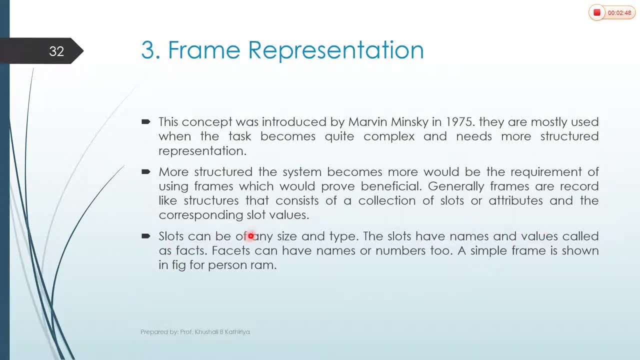 value called as a fact, okay, the name of the slot or the value of the slot, what we call it as a fact, okay. fact can have names and number too. okay, it may be a number, it may be a name, okay. so we can say, like slot have a number and name, okay. 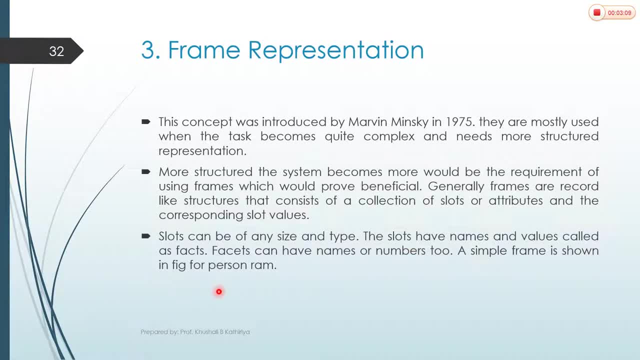 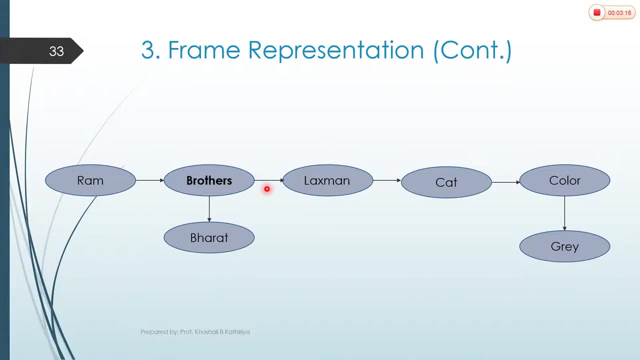 number or name. a simple frame is a showing figure for the person, RAM. okay. so first of all, here I give one example for the network representation. it is a semantic network representation example. here three brothers, RAM, Bharat and Lakshman, are brothers and cat color is a gray, okay. so here we have a 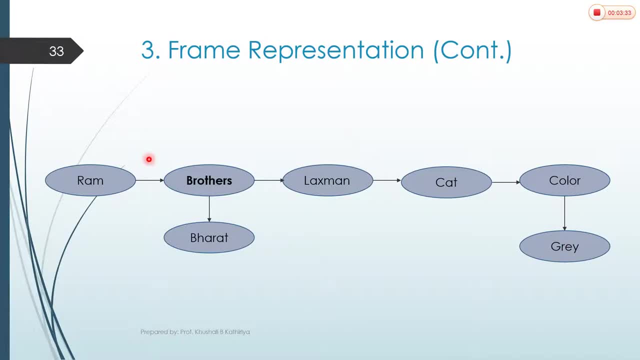 two sentences from Bharat and Lakshman are brothers and another is: the cat color is a gray, okay, okay, it is a representation for the these sentences here: RAM brother, Lakshman and Bharat, if this one is, are the frame? okay, I'm cabal. they both a school frame, both a little slot be both secure frame. be. 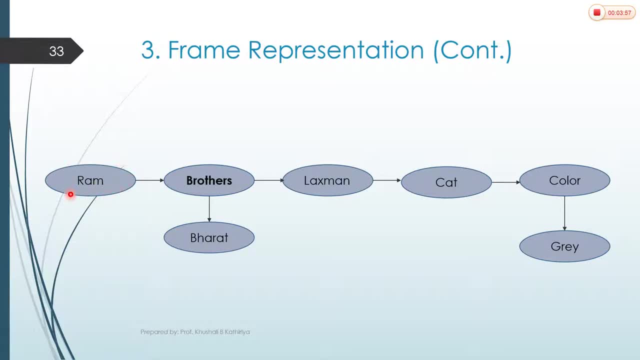 both of you, okay. yeah, well, you Joanna Ram K, a up entity bull. then software engineering made your entity attribute while I turn on to the peer. but entity has an Park, Yous Ми L overly modern game. I use firam used möra slot code. he present continental ticket. so here, Ram Bharat, Lakshman and brother. 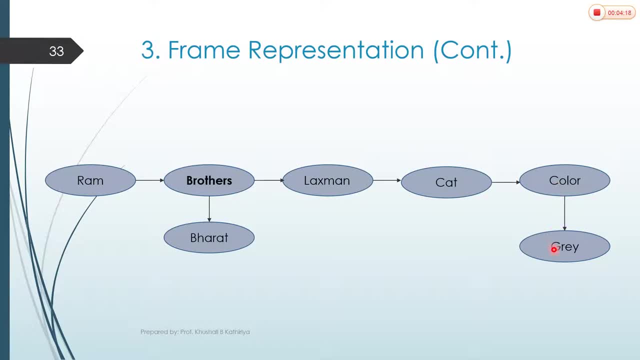 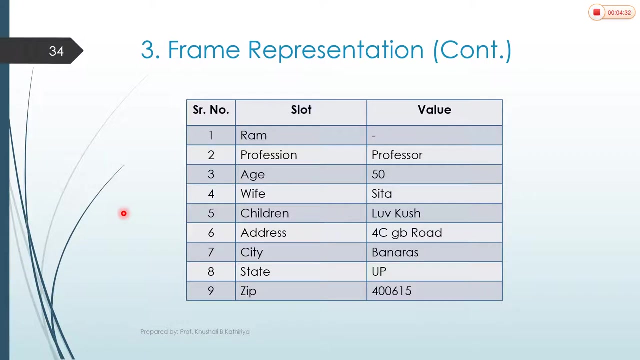 these are the fact. it color and gray, also fact. so here we represent our name, our number or value using soul, using a fact. okay, i give one frame representation example. here slot value are represent as a number and value may be represent in a number or name. okay, so here these are the serial number, simple. first of all, we have 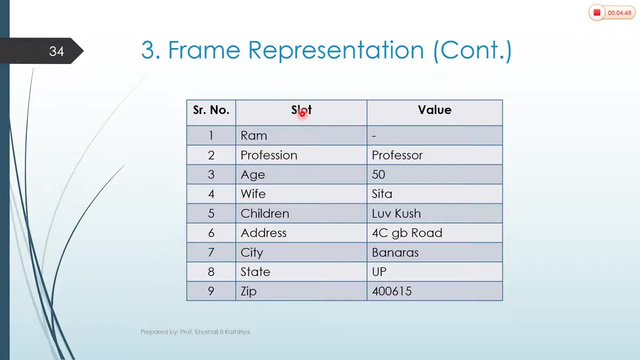 a first slot. first slot it means first frame. okay, so our slot name or our frame name is a ram, but ram is itself a value. so if they have not any value, another thing is a slot 2, it means frame 2. okay, so this is a profession. what is the profession? profession value is a professor. 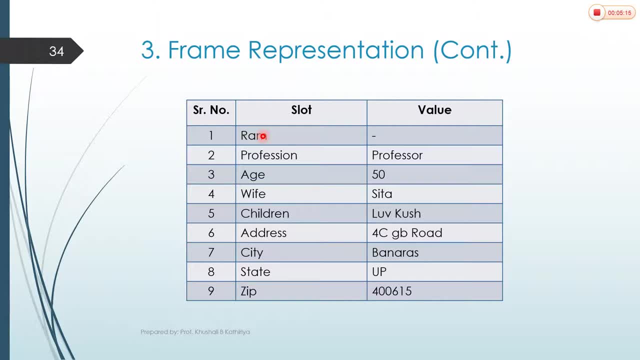 ram is a professor. so if we want to represent our data in or our sentence in, a network, represent on semantic net representation, then we have a two entity: first entity is a ram and second entity is the professor, then we have two entities: first entity is a ram and second entity is the professor. 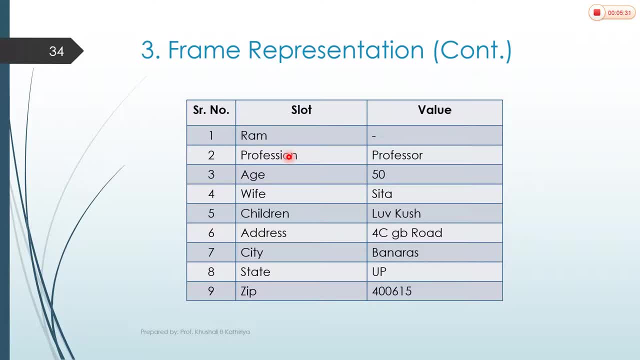 professor and from the link using a profession: okay, ram, profession is a professor. okay. another slot is the age. age has a value as a 15. okay, wife, sita, children, love kush. address 4 cgb role city is a bananas state is a up and zip number is a number. so here this one is. all are the slots we 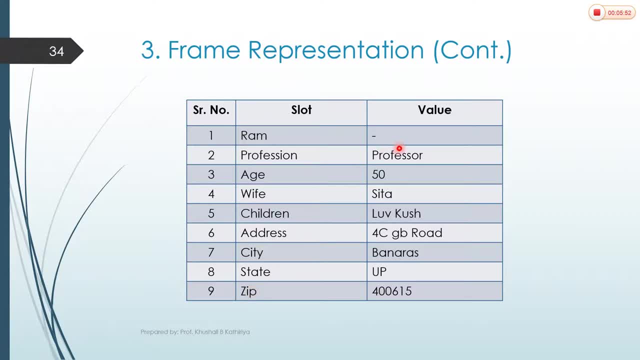 can also say, like a frame: okay, and this is a value of the frame, value of the slot, okay, okay. so this is a example for the frame representation. it is a simple example for your frame representation where, when we have a large amount of the data or large amount of the sentences are available and 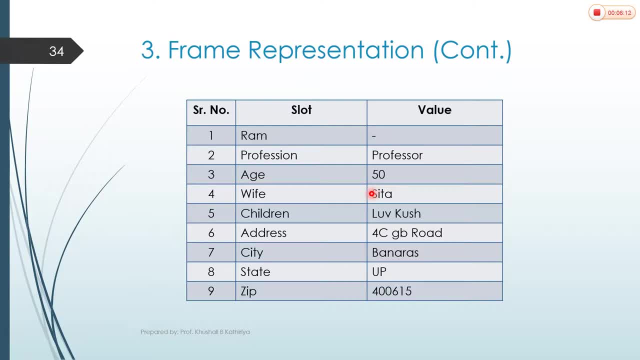 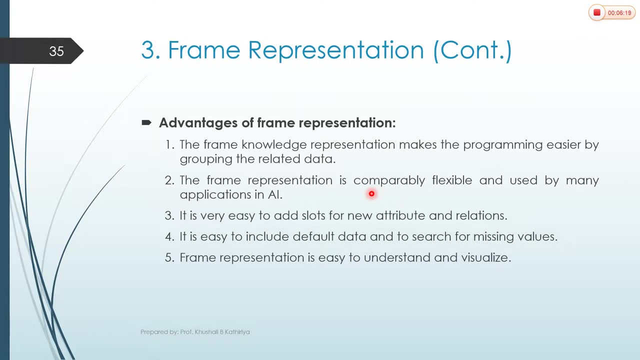 we want to structure this kind of the data, then we used a frame representation in AI. okay, so what is the advantage of the frame representation? frame representation, frame knowledge representation- make the programming easier by grouping the really like related data. when we want to relate the or grouping the particular data, then we use a frame knowledge. 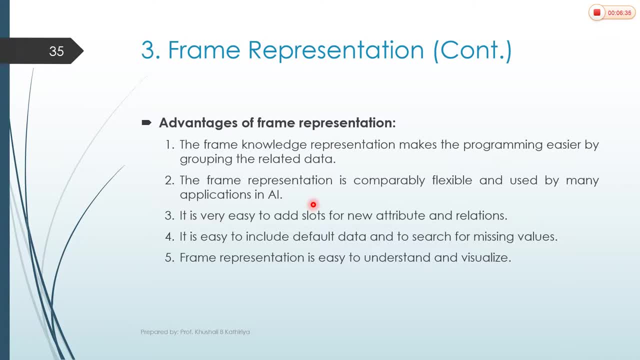 representation frame representation is the comparably flexible and used by many application in AI. okay, it is a flexible and used by many application. it is a very easy to add a slot for a new attribute and new relation by because we only have add new serial number, slot number, slot name. 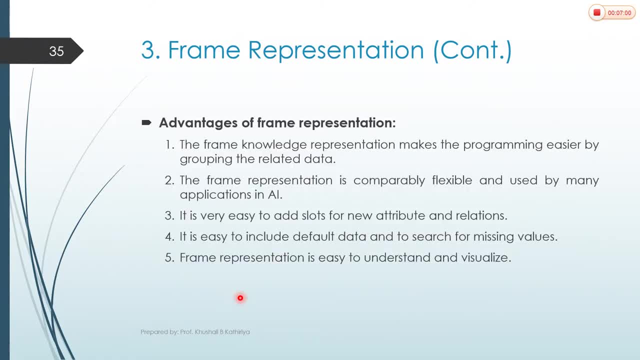 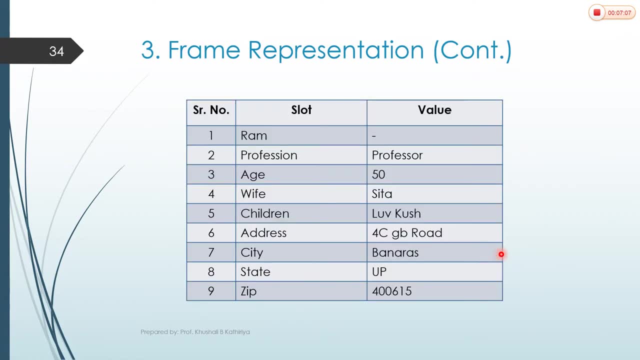 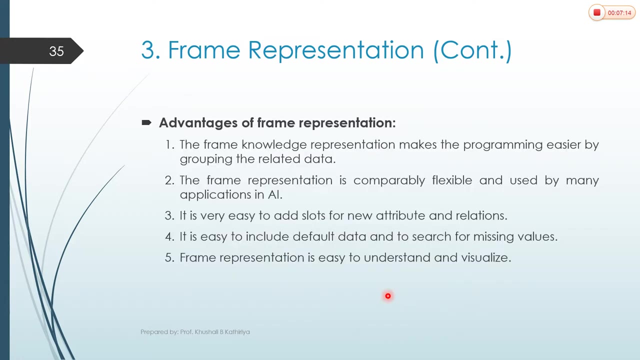 so it is a quite easy for the new attribute or new relation. it is easy to include a default data and search for the missing value. if any data is a missing in our slot value then we can identify easily identify from the frame representation. frame representation is easy to understand and